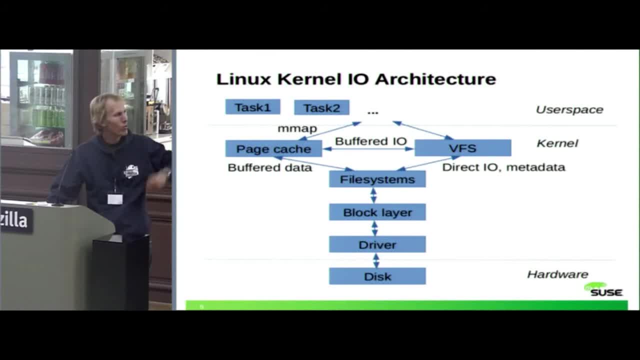 interface to do VFS, which is just generic Generic Unix name for the generic file system layer, Or you can do it via M-Mapped IO. so basically you M-Map and basically bind some parts of your virtual memory to files on disk. 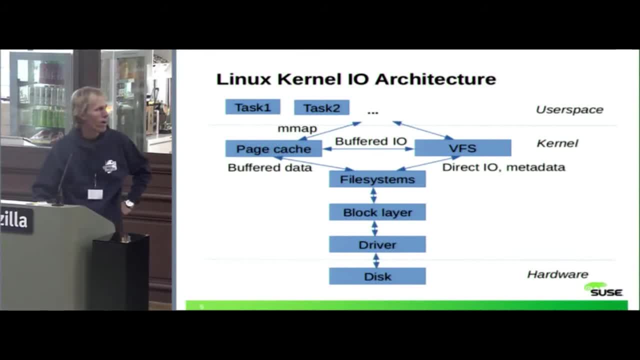 and then, just by writing to this memory, you actually write to the files. So then you go directly into PageCache, which is caching contents of the files on disk. Then either PageCache and VFS talk to the individual file system drivers. Okay, Okay. 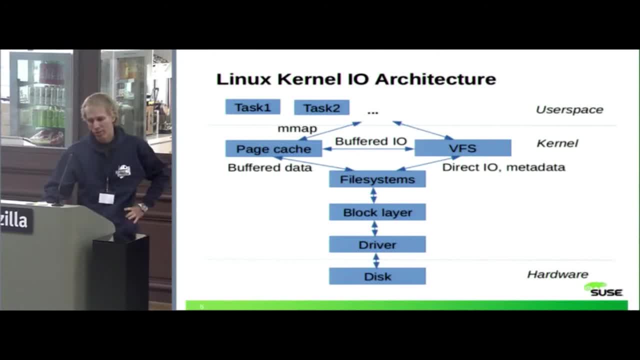 Okay, So these are the file system drivers which basically define on disk format, so how the data is stored on disk. They define what are directories, how they are stored on disk and they define access permissions and a lot of stuff like that. Then these file systems talk. 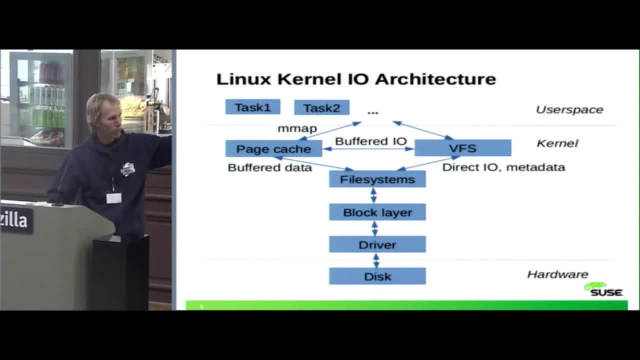 to block layer. so they ask it questions. like you know, give me block this or read that many blocks from this offset on and so on. And block layer talks to the device drivers and device drivers talk to the device drivers And device drivers talk to the actual hardware which then returns the data. hopefully, 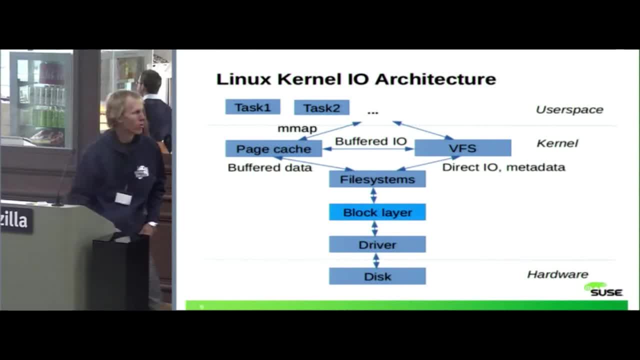 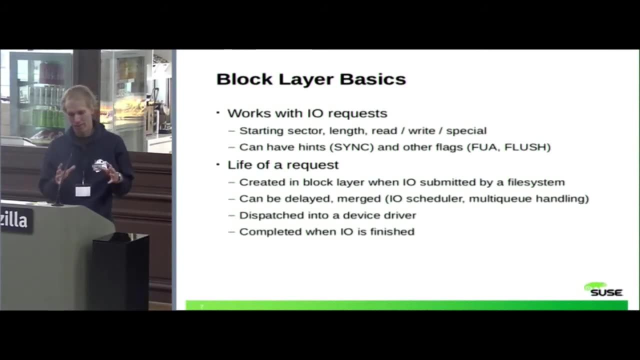 Now, basically, I will concentrate mostly to the block layer which is here and some of the old departing stems, but only to a small extent. So some basics. So block layer works with IO requests, so it's also about handling and shuffling IO requests here and there. 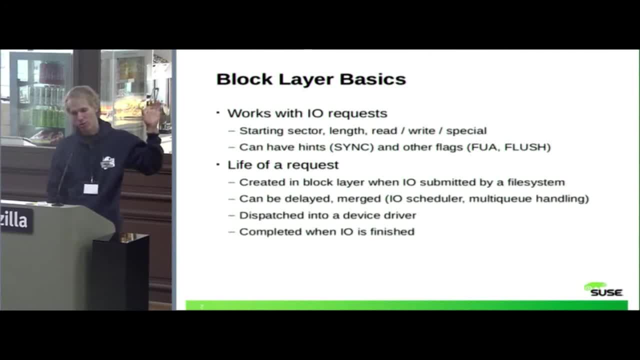 IO request is a thing which has a starting sector and length. It can be read, it can be write, and there can be also some special IO requests which do not carry any data. So these are, for example, like requests to discard part of the media. 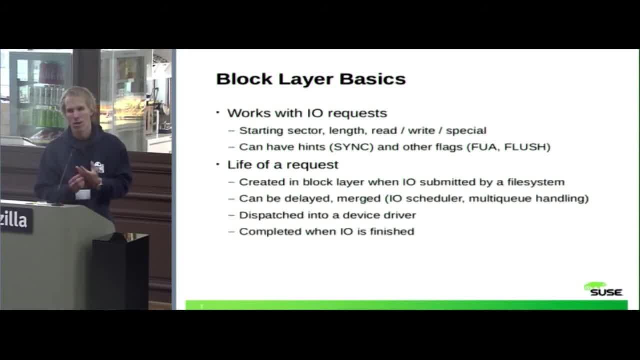 For example, this is usual for SSD disks where you have discard operation, or it can be a request to flush write-back caches or so on. So that's also handled as an IO request. but it's kind of special because it doesn't have any data attached to it. 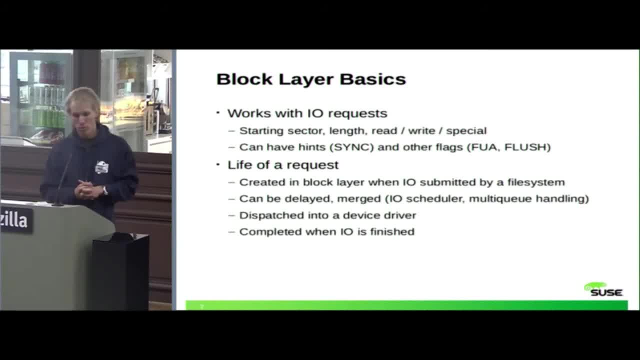 Each IO request can have also kind of hint attached to it. So example of a hint is that the request is actually synchronous, which means that someone actually waits for the IO to complete. So reads are usually synchronous, unless it is read-ahead. Writes are sometimes synchronous. 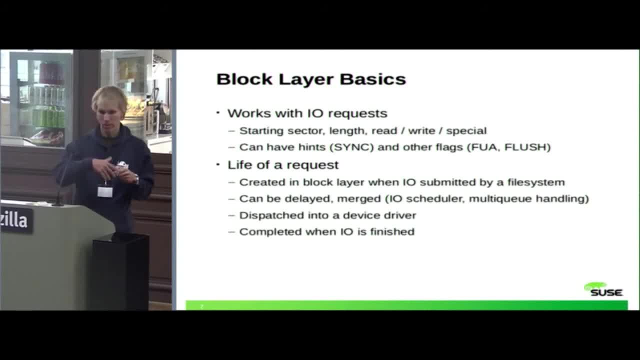 For example, when you call fsync, then you actually actively submit the data to the disk and wait for it to complete. Or when you use direct IO, then again you submit the IO request and wait for it to complete. They can be also asynchronous. 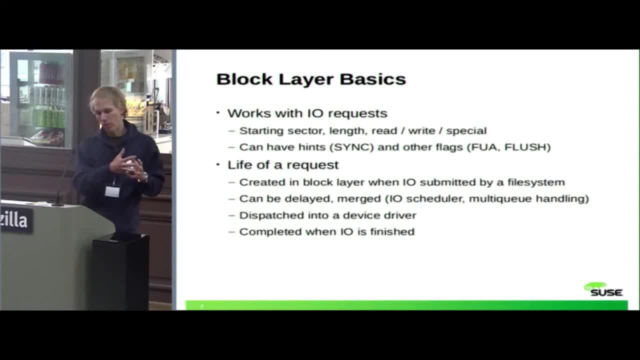 because when you use buffered IO, you just actually write the data into the page cache and then kernel, when it decides So, it will write back the data from the page cache to disk. So in this case no one actually waits for the write. 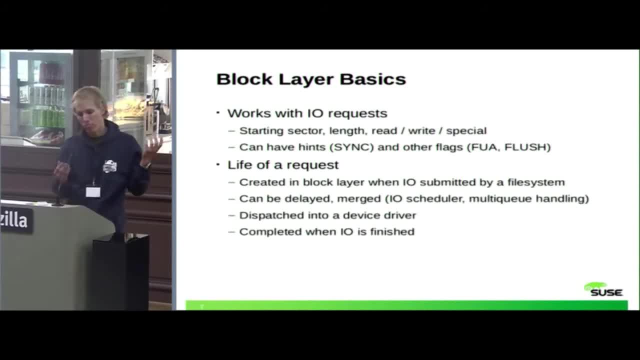 It's asynchronous, And so this hint may or may not be obeyed by the IO scheduling algorithms, and they may decide on the priority of each IO request based on these hints, for example, And there are some other hints, Then you can have also other flags attached to the IO request. 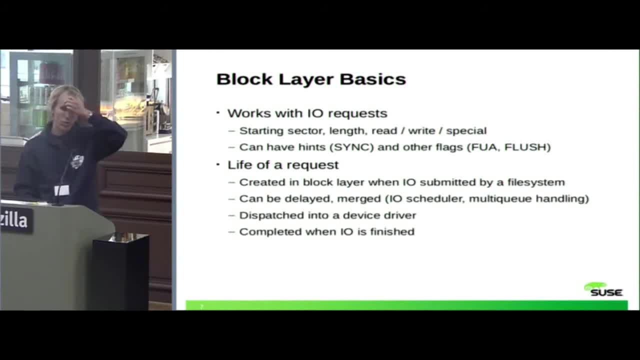 like FUA, which means force unit attention. It's a shortcut for basically saying: I really want this write to go to the media, I don't want it to be in a write-back cache. And then there are ones like flash, which I have talked. 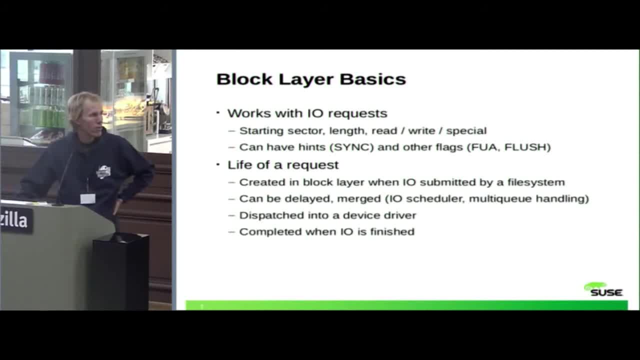 This means basically, before this IO happens, write back anything that you have in write-back cache to the media. So these requests are needed, for example, when you are implementing general link in the file systems and you really want to make sure that the data makes it. to the stable storage and is not just in some write-back cache on the disk itself. Or especially if you have clever storage, they can have gigabytes of memory in them actually. So usually they are battery-backed but they are not in the stable storage. 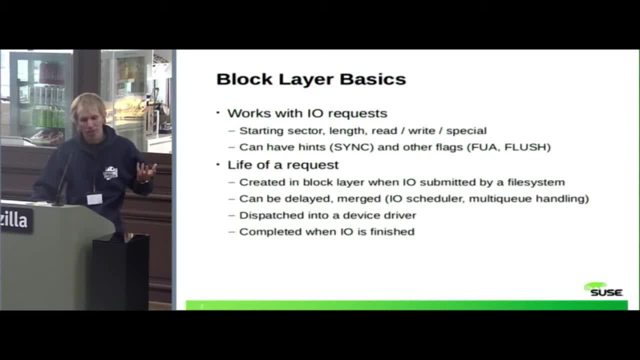 So that's why there are these. And on standard SATA drive the cache definitely is not battery-backed, So each IO request goes through several phases, So it's created in the block layer when the file system requests some data or sends some data to write. 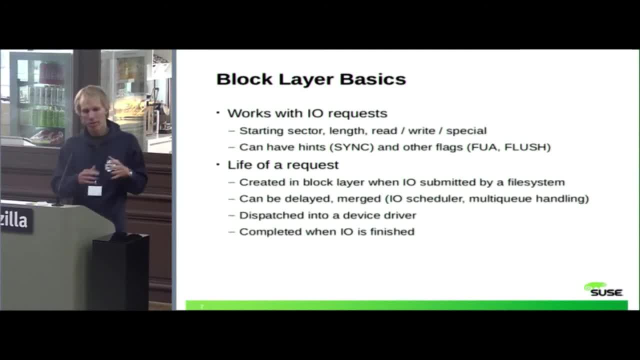 Then it goes into IO scheduler where IO scheduler decides this request can wait. This request should go to the driver. It can be merged with other IO requests because they are actually consecutive And then its advantage is to actually merge them in one larger IO request. 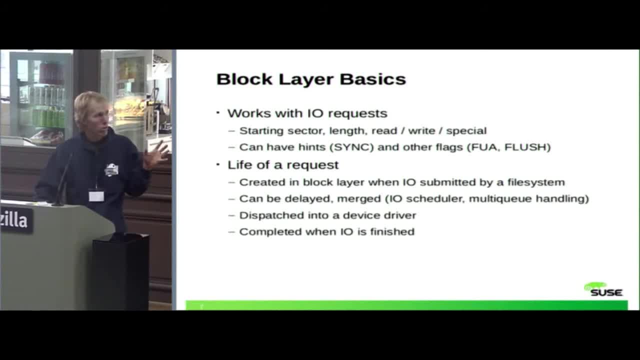 There is also for especially fast devices, this IO scheduling actually doesn't happen. There is something which is called multi-queue handling, but we will see it in more detail in another slide. Then, eventually, when the IO scheduler decides so, or when it goes through the multi-queue, 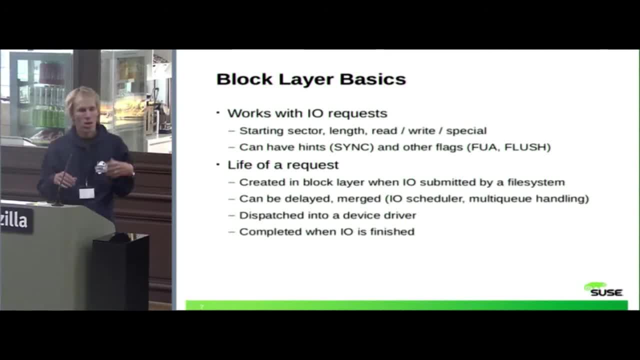 the request is dispatched, It goes into the device driver And device driver just directly submits it to the hardware. Hardware eventually signals that the IO is complete via interrupt And then we call some callback of the file system saying okay, now the IO is finished. 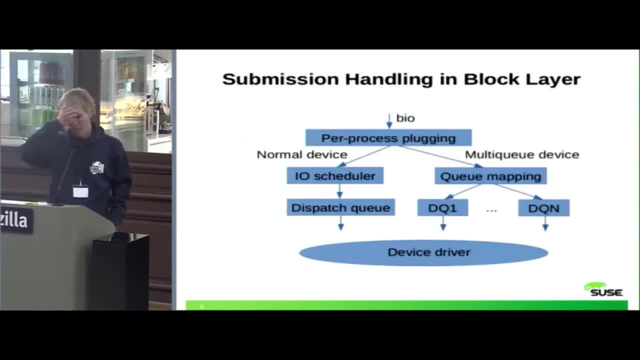 Do what you want. So here is the block layer in the detail. So from the file system comes a structure which is called bio. It basically has again offset length, some pages attached and some other information. Now first, actually when the file system 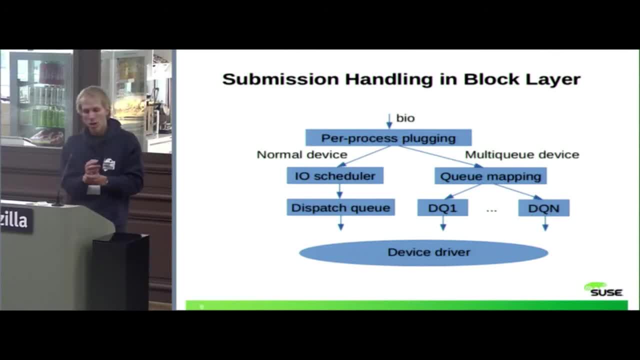 submits such bio structure, it is added to a per-process plug list, so-called. So each process has a list of outstanding IO requests. When you start submitting IO, we say that the process is actually blocked, which means that actually we are delaying the request for a bit. 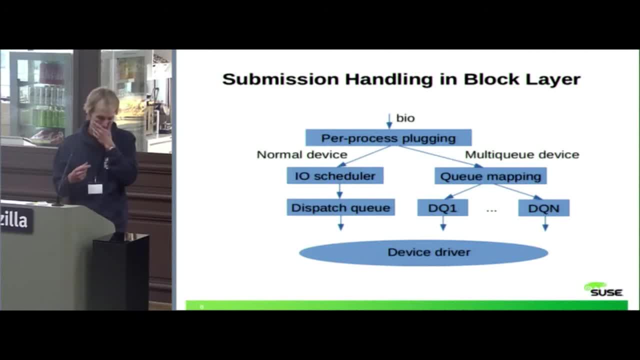 awaiting whether they could or whether they could be merged together. So usually the experience shows that when you delay requests for a bit, you can find quite some opportunities for merging requests. So we delay these requests and either when there are more than 60 requests accumulated. 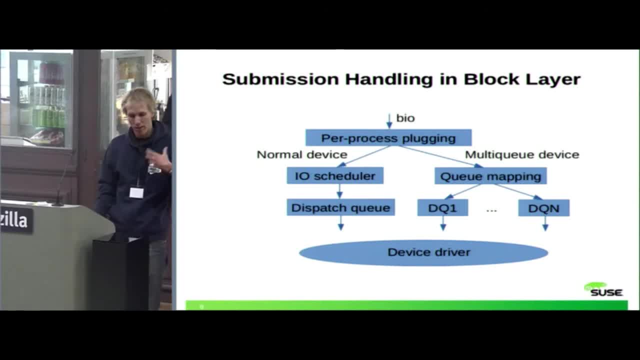 or the actual bound, doesn't really matter- then we flush the list and start again. Or when the process goes to sleep, like for example when it wants to go to sleep or when it wants to wait for the IO- we will flush the plug list. 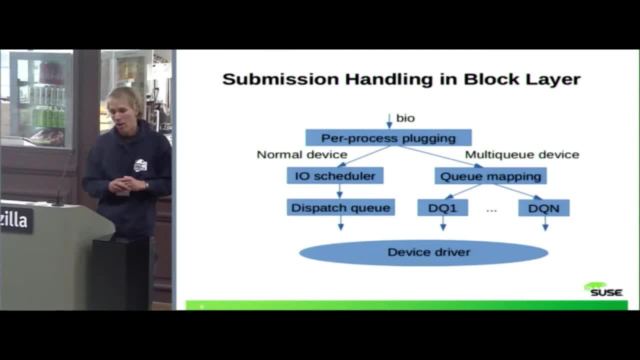 and actually submit it further into the block layer. Now then, when the request eventually so when the process plug list is unplugged. so we will submit the request either to the IO scheduler, which does some decisions on ordering of the requests. 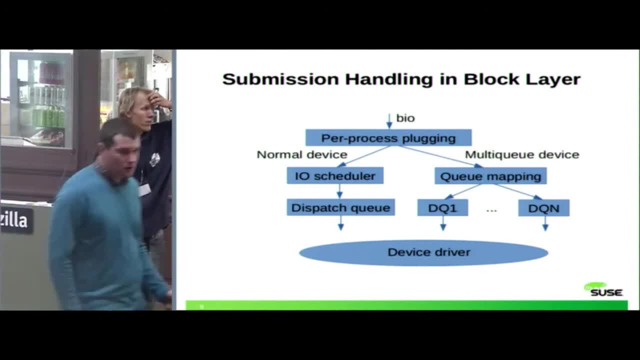 and so on. And then, when the IO scheduler decides it's time to send the request further, it will be added to the so-called dispatched queue. Now, this is the like standard path. It was used until recently for all devices. 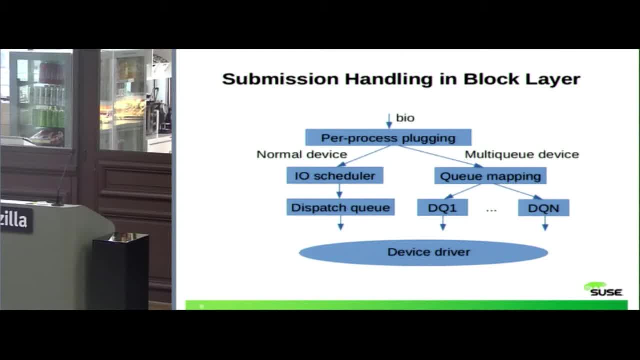 Now for the really fast devices like PCI-E or similar devices. we have now one thing which is for booting and handling, So that's like really fast. It's a low overhead path For devices. it also allows for multiple hardware use. 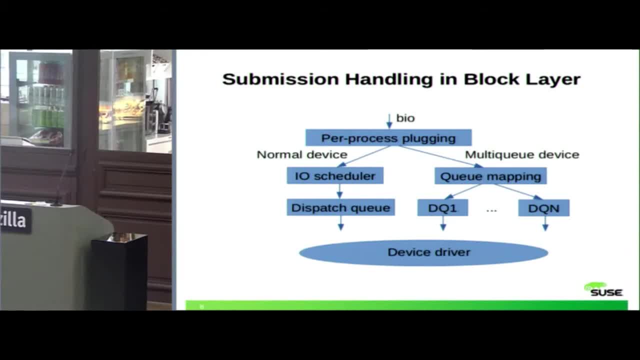 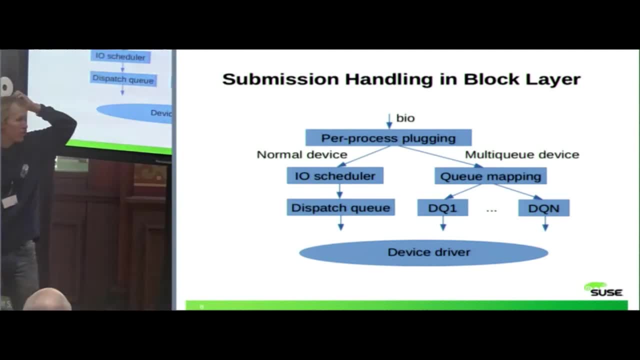 And there is no IO scheduler. it's really just you decide which hardware to send the request and then use some device driver. Now, the answer to the thought about this part will be in the next talk, so I won't go into much detail there. 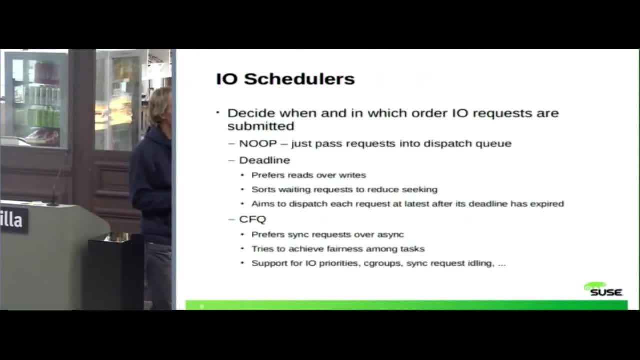 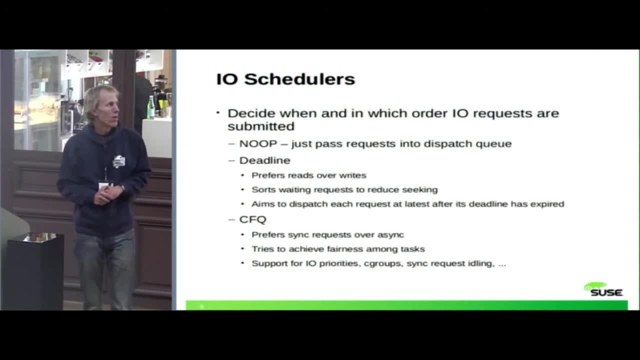 So what happens actually in the IO schedulers? so there are three different IO schedulers in the kernel. So there are three different IO schedulers in the kernel. First is no-op and that's a simple one that basically just passes the request directly. 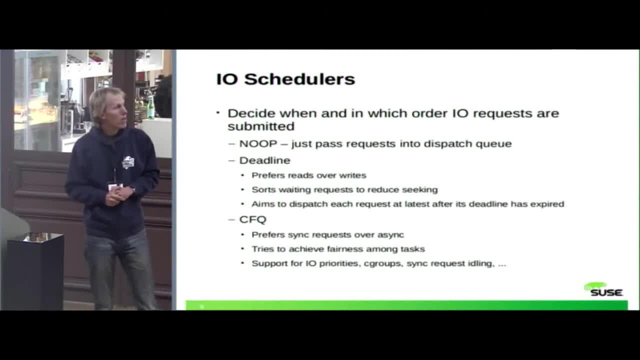 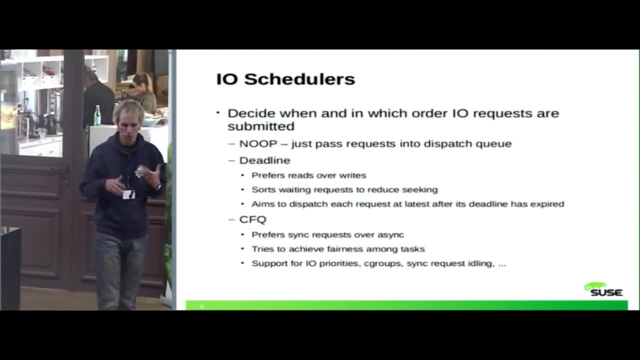 into the dispatched queue. it does no decisions. Then there is deadline IO scheduler, which is kind of middle ground. So the idea behind IO scheduler is that deadline IO scheduler tries to prefer reads over writes because reads tend to be more difficult to get observed. latency of the system. 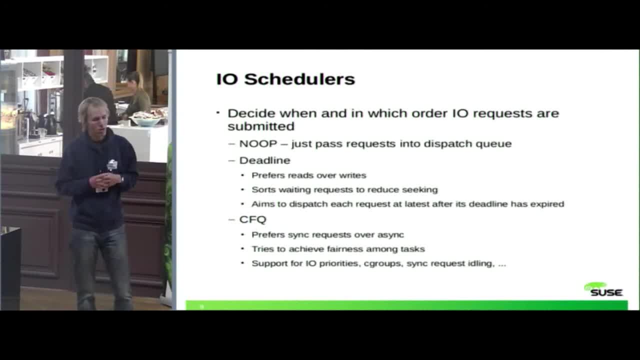 and the experience of the system. So when you submit a read, then it tries to dispatch it, Or when there are outstanding reads, it prefers to serve these reads against serving writes. But there are some rules so that writes aren't starved. 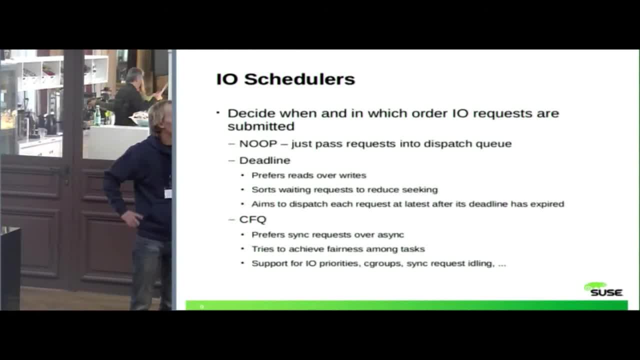 that much, I won't go into that now. And it sorts all the incoming requests by the starting sector. So, like, all the requests that are waiting for now are sorted and when you submit a new request it's checked whether it can be merged. 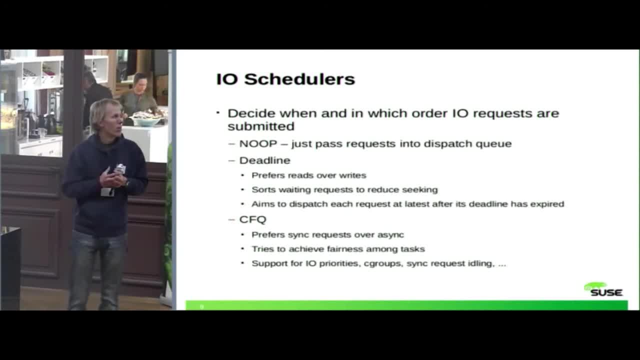 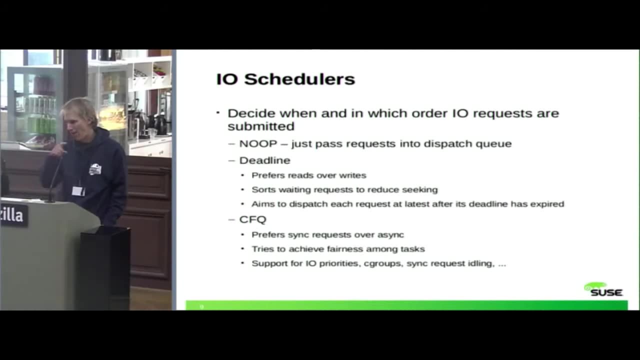 to any of the outstanding requests And, oh sorry, And it aims to dispatch each request until the deadline expires, So each request is assigned a deadline. Now the deadline is different for reads and writes, And it tries to, and when the deadline actually passes. 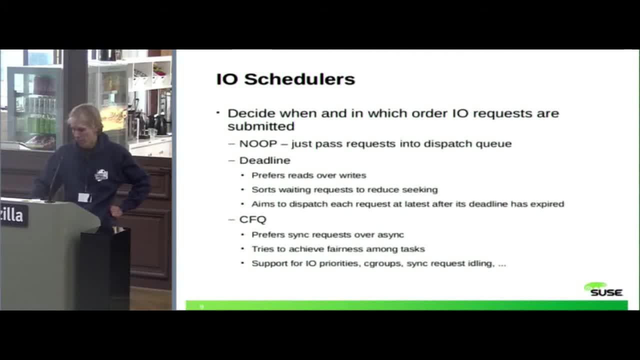 it's given really high priority and basically it's then submitted as soon as possible to the device driver. Now, the most complex IO scheduler is CFQ. It supports a lot of features like IO priorities. okay, Like IO priorities, so basically you can assign priority. 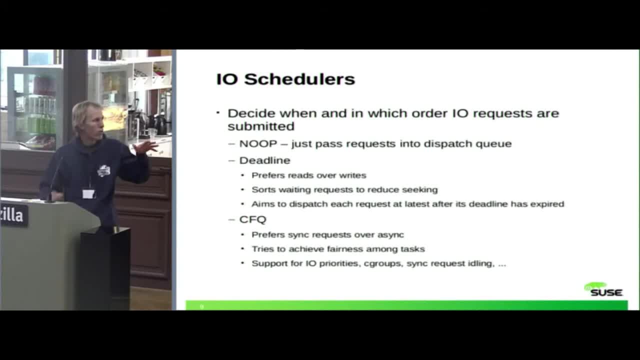 to each process and then the process. then the scheduler tries to schedule requests, So to achieve some kind of fairness among tasks, So each task is supposed to be given same amount of same amount of time on the disk, Or and IO. priorities now modify weights. 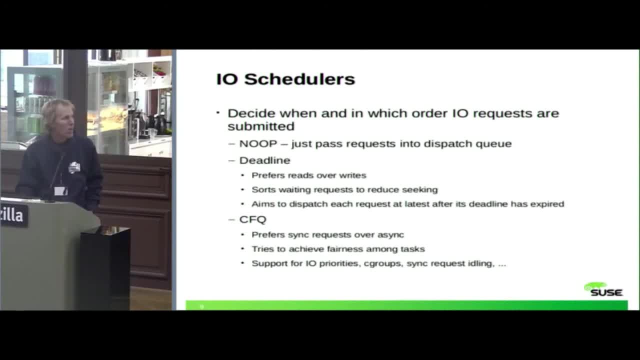 so process with higher priority is given more time. In CFQ scheduler it's a little bit different. It's also support for C group. So basically you could limit, you could give a proportional share of the disk bandwidth to a different to each C group. 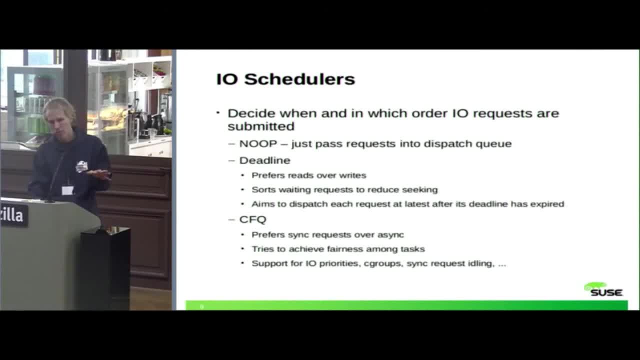 CFQ actually doesn't distinguish between reads and writes. It rather distinguishes between synchronous and asynchronous requests. Now, as I already said, reads are mostly synchronous, Writes are sometimes synchronous, sometimes not. That depends. And it has also other features like synchronous request idling. 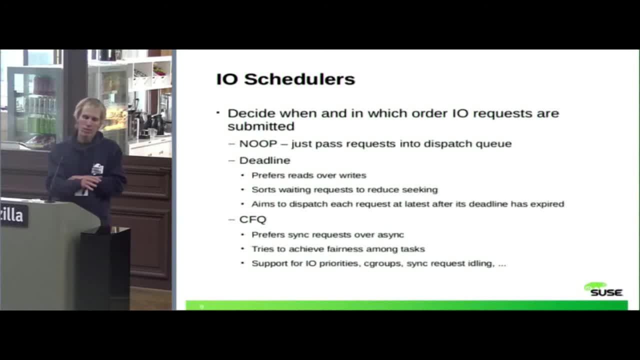 which means that basically, when the process submits synchronous requests, then the CFQ will wait and won't give the throughput to and won't basically schedule IO from any other process for a while after this request, after this process stops submitting and it waits. 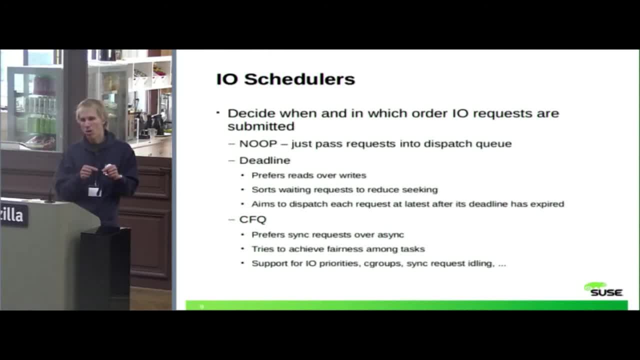 Whether the process actually won't submit even more, or synchronous IO, And the idea behind this logic is that usually these synchronous requests are related, so hopefully they will be close together on disk, So this is some way to also improve user experience. 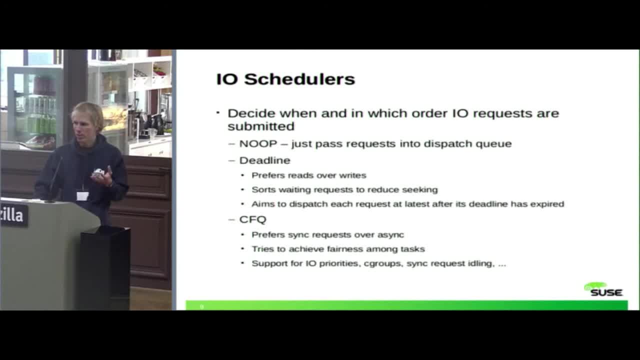 On the other hand, basically you have there periods of time where the disk is actually sitting idle doing nothing, because the first process doesn't do any IO and you don't allow any other process to do IO yet. So it can result in really an error. 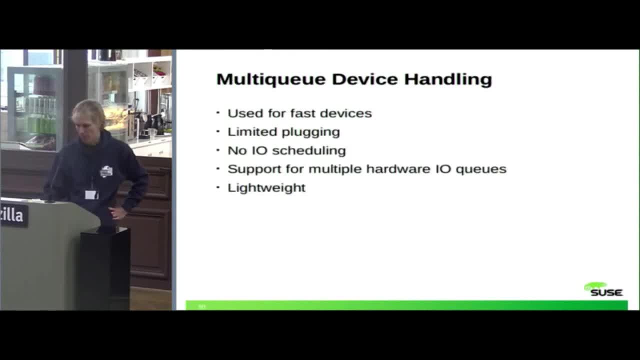 It can result in reduced throughput in some pathological cases. Yeah, Is it up to the scheduler the download of the device to support the MCQ? Yes, the scheduler will find out whether the device supports MCQ and so basically, MCQ means that the device 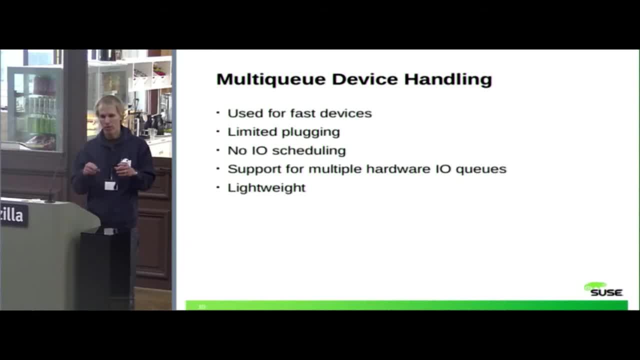 can support more IO requests running in parallel. Normally, then, you just submit one request, or that's the simplest case: You submit one request, you get the result, And so on. supports NCQ. it means that you can submit more requests. 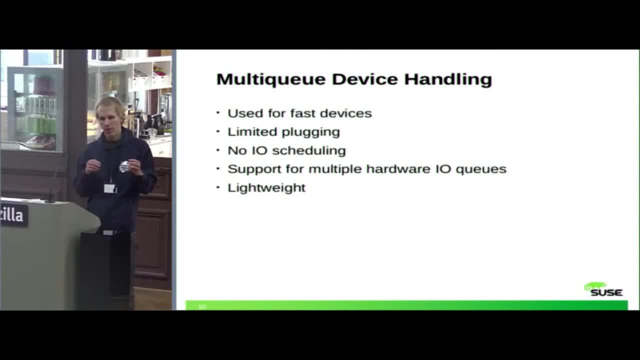 each request is assigned something which is called tag and then basically that's identifier of the request, so that the driver can actually tell to you which request was completed and so on, And so the block layer will actually find out whether the device supports NCQ or not. 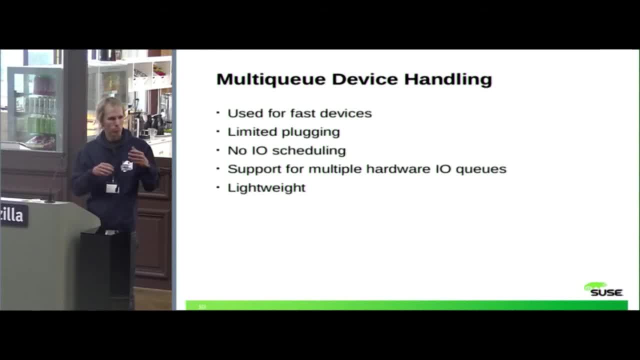 and it will assign tags to IO requests and then submit as many requests as there are tags basically. And there is also some logic of assigning tags which is most important for the multi-queue devices, for the, because there it's hard or there it's not trivial to do it in a lockless manner. 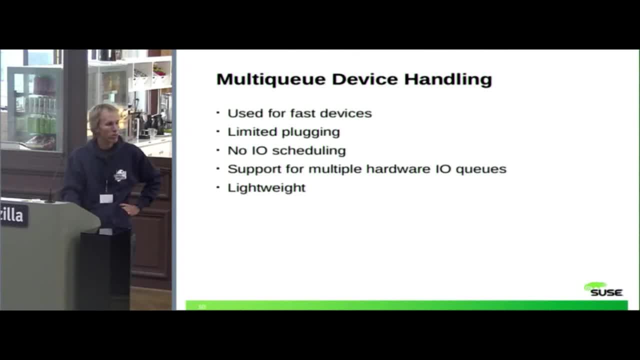 but for normal devices it's basically done under lock and their logic is relatively simple. Yeah, So multi-queue device and link, as I said just briefly, it's used for fast devices, devices which have more hardware queues. it's a similar situation that has happened. 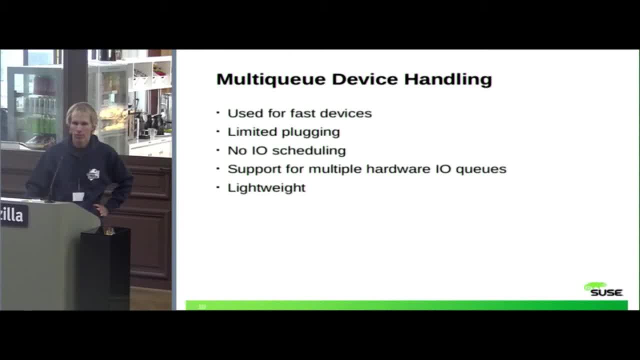 in networking space a few years ago. So basically, to drive the heavy parallelism within the device, the devices already have to expose that there are several independent queues. there can be several independent queues of IO requests and you can queue these requests to several hardware queues. 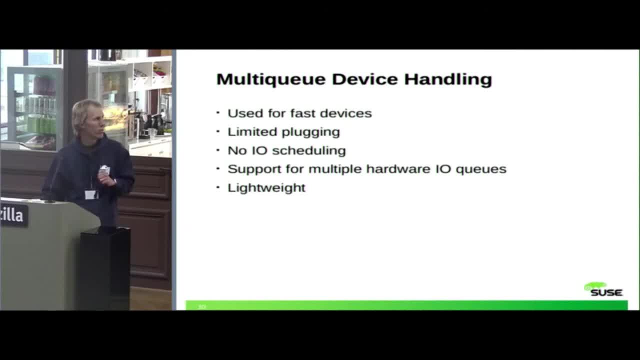 Usually they are bound to different CPUs, so that you can maintain some CPU locality and thus reduce cache bouncing and stuff like that. Yes, that We do no IO scheduling for such devices. there is only limited plugging where we just maintain one request in the plug queue and when. 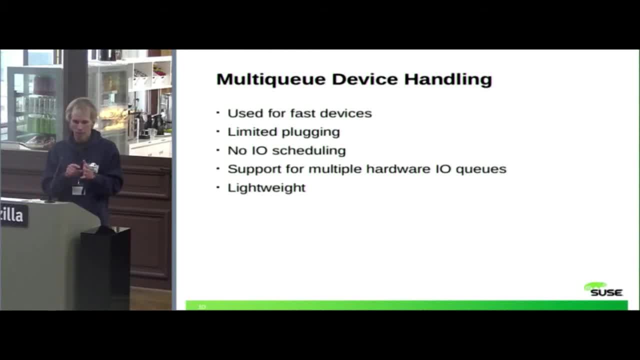 another request arrives, we just try to merge it with this request. If it can be merged, then good. if it cannot be merged, we flush the first request to the device and attach the new requests into the plug queue. And it's very lightweight, completely lockless. so on. Jens will talk about the details, so I won't spoil his 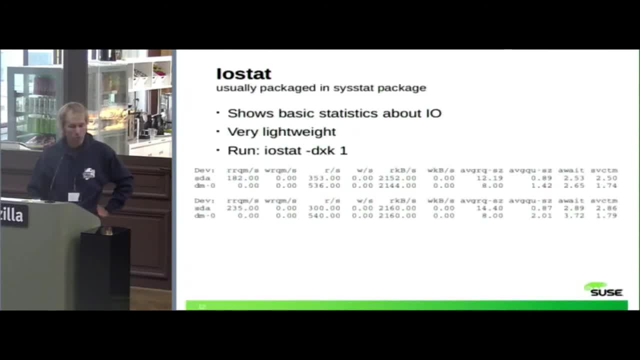 talk Now tools you can use for performance analysis. So the simplest tool is IOstat. I guess some people know it here. It's part of a sysstat package in the distributions and it shows basic statistics about IO. It's very lightweight so you can use it without the fear that it will actually. 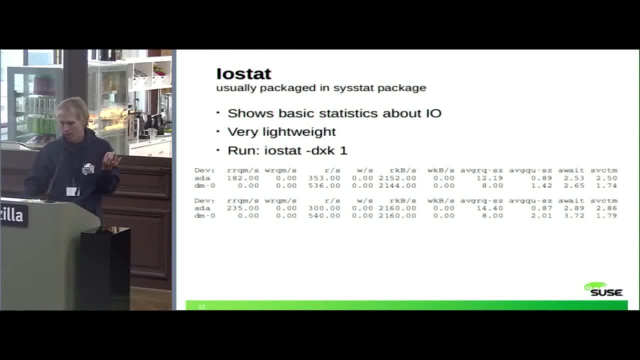 interfere with the workload you are running. So below is an example of how looks output from the IOstat minus the xk1.. One means that basically every second the statistics are printed and in the first column you can see the device name. So these are actually results for two consecutive runs. First, 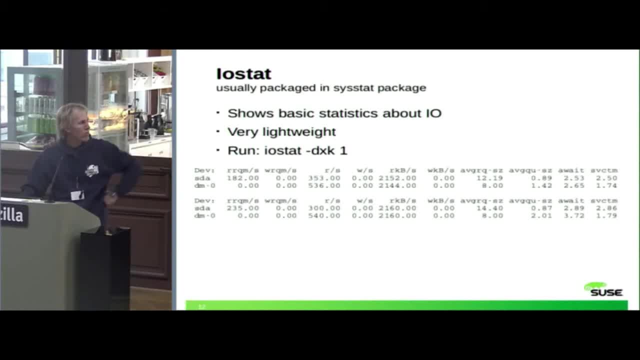 this device name. then there is then two columns show number of merges per second, 00urt second. the further two columns show number of reads per second, number of writes per second and how many kilobytes were read and written per second. Then average request size. that's in sector, so we can see that there were like six on. 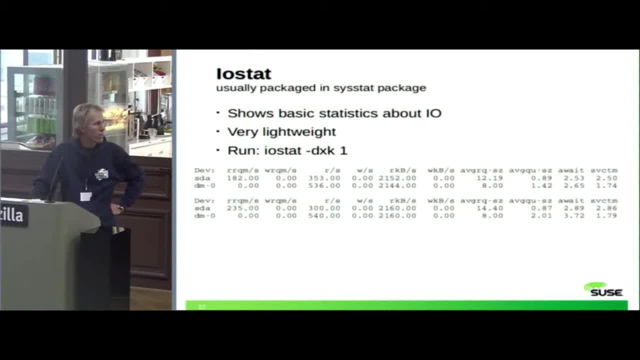 average six kilobytes in each IO request for the SDA device and four kilobytes for the DM device. That's one thing. to bear in mind that actually for device mapper devices these numbers are kind of bogus because they don't do real IO scheduling or IO submission. the device: 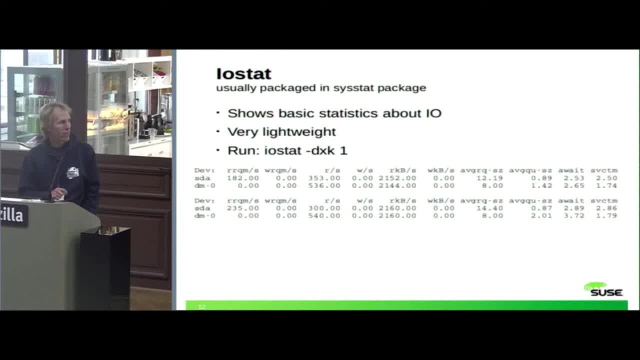 mapper devices just work with BIOS and so, for example, request size is always just four kilobytes, because that's the page size. The real merging and IO scheduling stuff- very interesting stuff- happens only for the real devices, like SCSI devices and so on. Then average queue size is the next column. that basically shows how many requests are. 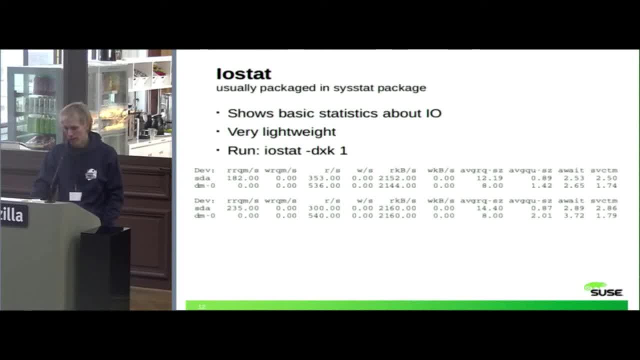 waiting In the queue before they can be submitted to the device. then we have average wait time, which is: how long on average did the request spend in the queue before it was submitted to the device? So how long the request was handled in the IO schedule? and these two numbers are in milliseconds. 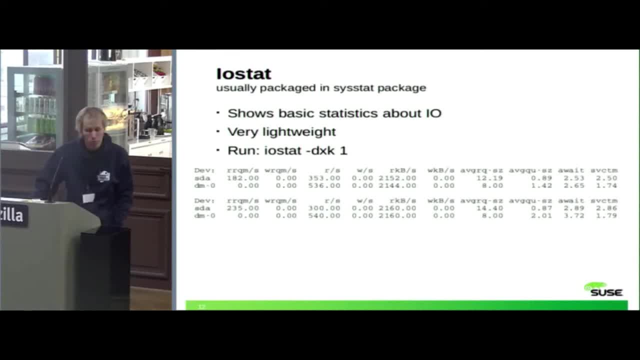 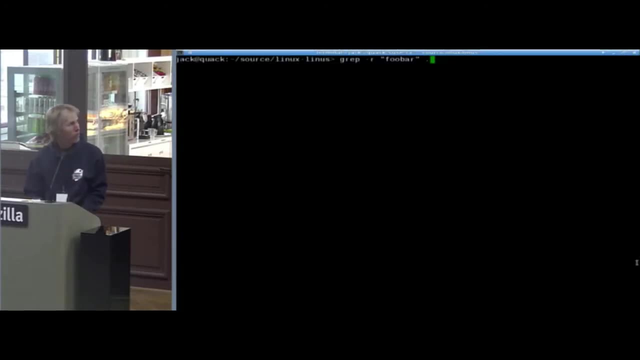 The third number, again in milliseconds, is service time, which means the time between the request was dispatched to the device driver. So this is how long the request has been completed. So here I have prepared a small demonstration. So here I will run some grep through the kernel tree, and here I will run iostat-dxk1 and here 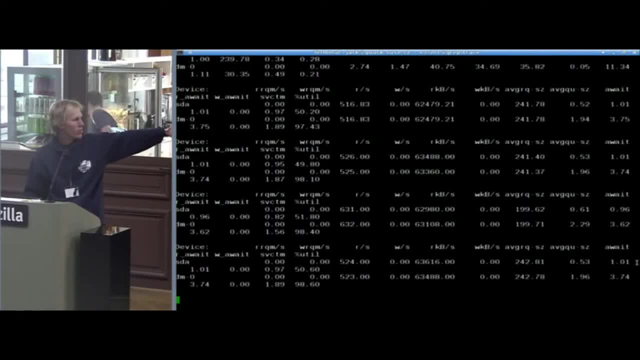 you can see that the disk is doing some 60 megabytes per second, So it's SSD SBR greping through the kernel tree. The request sizes are relatively small and you can see actually the smaller the request, the slower the IO goes. So we can see it works and if I stop the search then you can see the numbers have dropped. 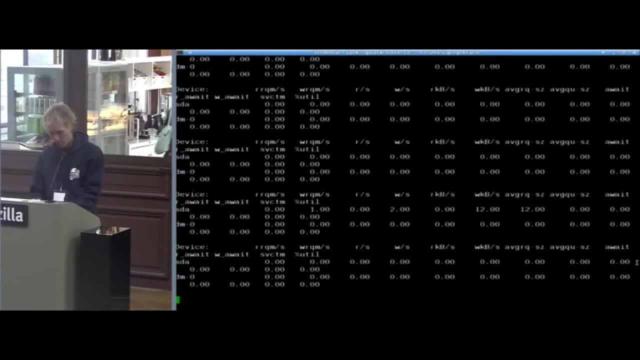 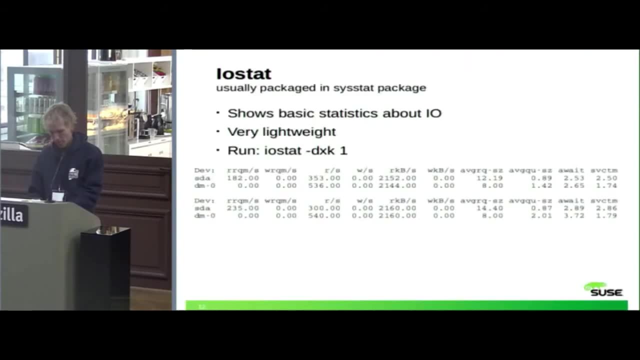 almost to zero. Occasionally there is some read or write basically of like changed 8 times or so on, but nothing really happens anymore in the system. So that's a simple tool to use and usually you start when you are investigating some problem. you start looking at iostat data whether there isn't something suspicious, and even 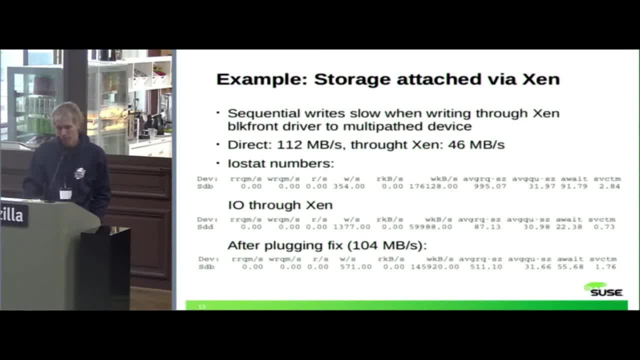 though the tool is simple, you can already debug some problems with it quite successfully. So, for example, here is one real customer problem. They found out that when they access the storage through Xen block front end driver- and it's kind of important that the device was actually some multi-pass storage or going- 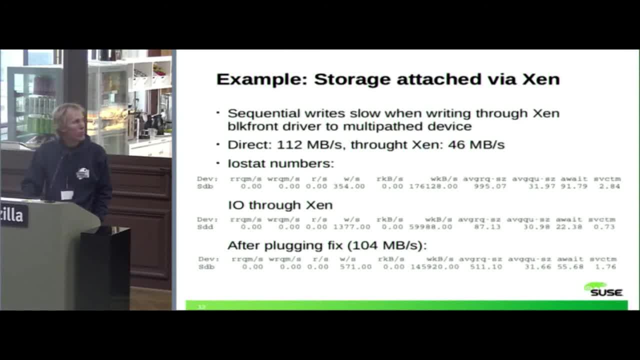 over fiber channel, then the throughput is quite bad. So it was sequential write and when you went directly, the storage was doing some 112 megabytes per second and when going through Xen it did only 46 megabytes per second. so it was big difference. 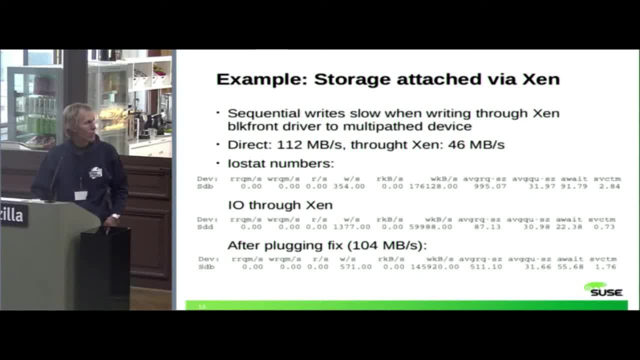 So they were kind of wondering why that is So. if you look at iostat numbers, the first numbers are for the direct access and there you see that we are doing a lot and the request size is actually around 500 kilobytes. So one IO request has around 500 kilobytes. when you are going through Xen you will notice. 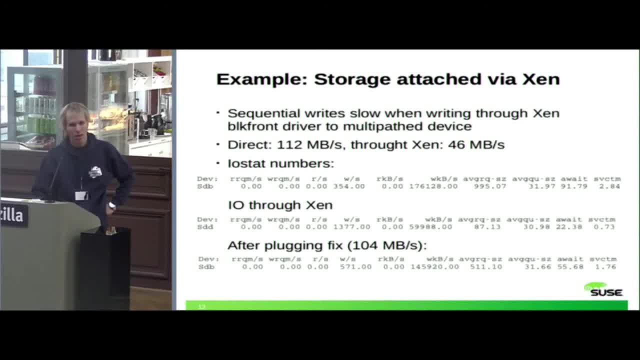 that the request size is actually only 40 kilobytes and that's due to, if you look into why. So one thing to know is that basically, when you submit small request like that to the IO storage, then usually the throughput really suffers. The storage achieves maximum throughput around those 500 kilobytes, even the megabyte request. 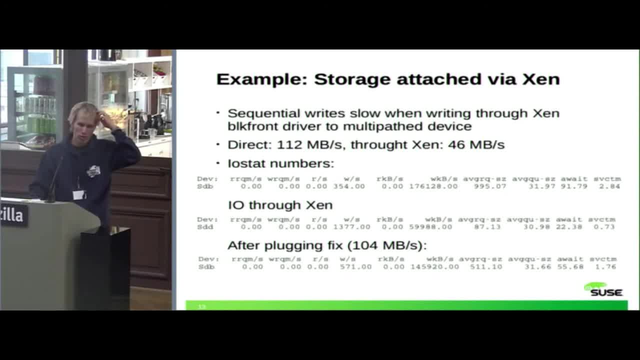 sets, where the storage is like with traditional rotational disks, achieve maximum throughput. So request size such as 40 kilobytes really make the throughput suffer. So that's one thing to know, Thank you. And the reason for it is some internal handling in the frontend driver of Xen where it didn't. 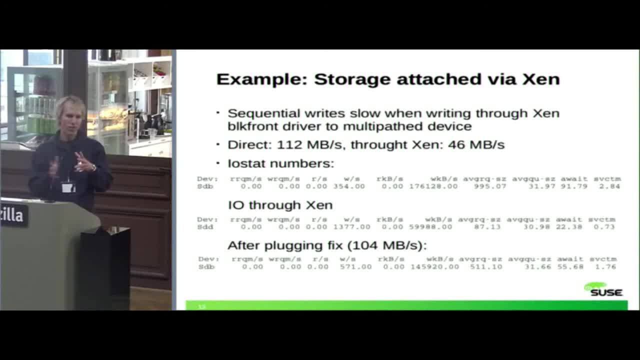 do any request merging and it was through some internal Xen bus going from Xen backend to Xen frontend. it was able to pass all the requests with just a couple of pages attached, so like 10 pages attached because they didn't have more space in the structure. 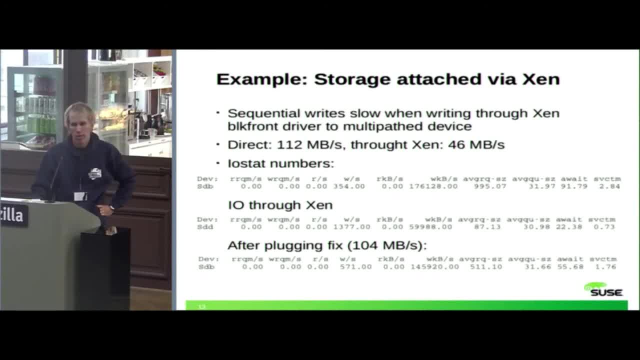 So when we did some, when we implemented some basic IO plug-in, Okay, In the frontend driver for Xen the request size increased to some 256 kilobytes and the throughput increased back to 100 megabytes. So it's still not quite as direct access, but it's much closer. 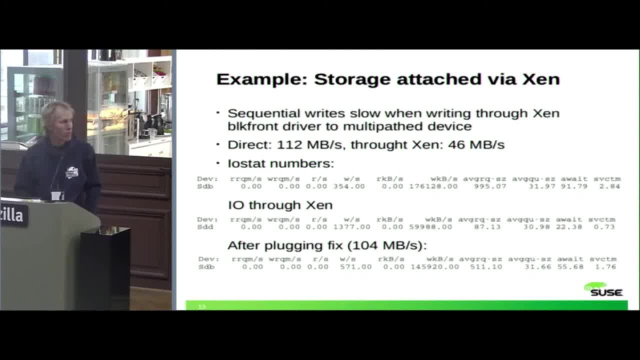 So that's, that's one of the example how even simple tools such as IOSTAT- yeah, so it's the IO. So if you run IOSTAT-DXK, it will just show this data. I don't know, I have. What do you mean by the? 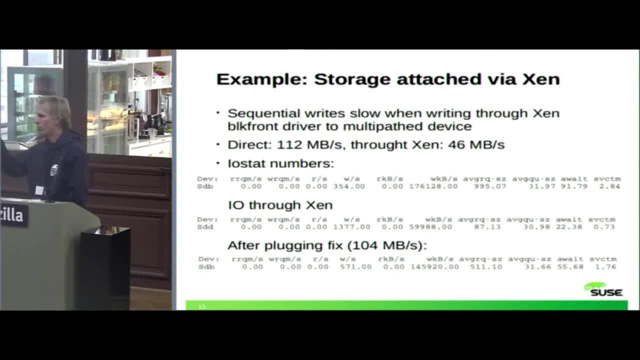 Yeah, it was just a file copy, or basically it was DD from dev zero to the device. you know that, that's that's so. they were obviously first they were looking a bit into what happens, you know, there, and we found that simple file copy already shows the problem. and then we 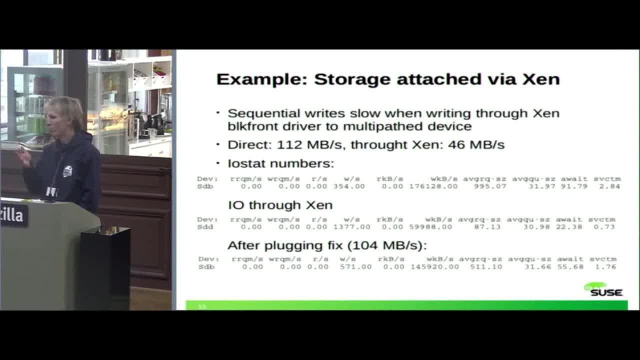 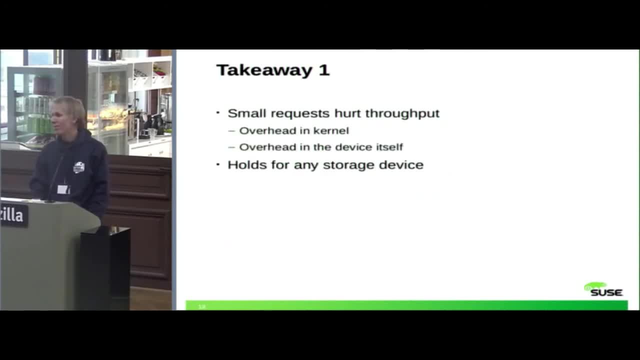 started online, then you have such a simple reproduction of the problem, then you can you realize with the tools, or you can, like you'll see in the last example, that it isn't always as simple. but yeah, this was a simple case and IOSTAT was enough to understand what's. 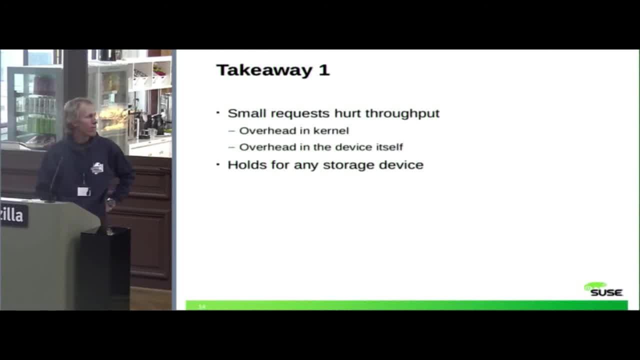 going on. So take away from this, from this first example, is that really small IO request hard throughput? a- because you have each IO request has some overhead in the kernel itself in the handling. b- because each IO request has an overhead in the kernel. Okay, 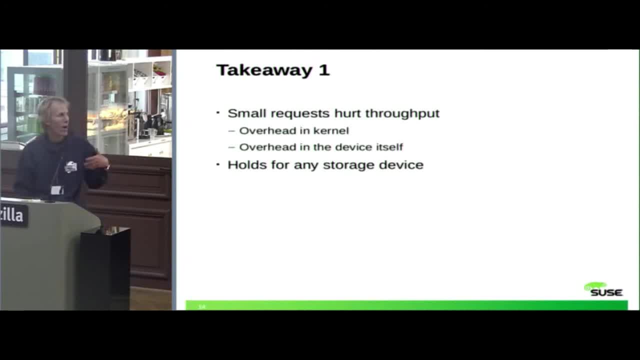 In the storage itself. so the smaller request, the higher is the proportion of this overhead and so the throughput suffers, and this holds basically for any storage device, regardless of the type, but to a different degree. so, like some devices don't suffer this as much. but basically you have to find out what's true for your device, because there are like device. 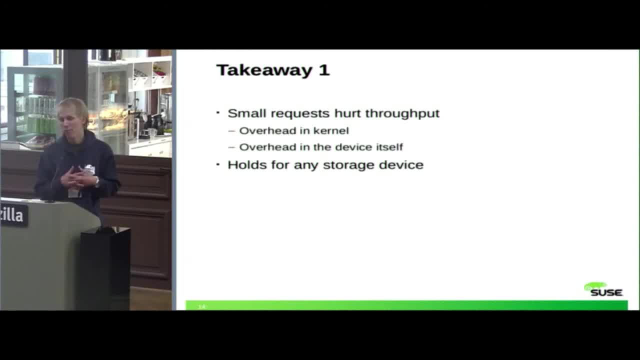 like storages. you would consider the same, but actually they behave quite differently. Okay, In presence of small requests. some are able to merge in internally, some are not, so depends Now, another tool is IO watcher. it was written by Chris Mason, the address where you can actually 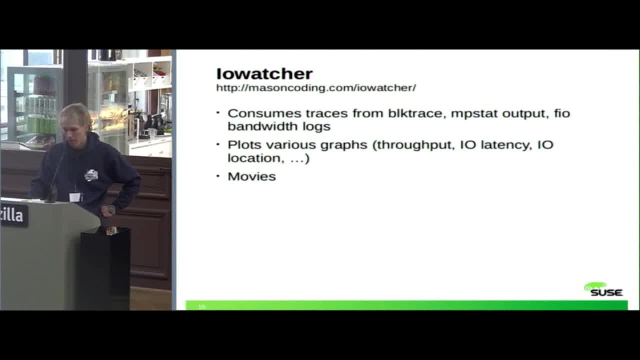 find and download. IO watcher is there. there is a git repo on kernel org also. it consumes traces from block trace. I will speak about block trace a bit later. it can also comes from block, so so block trace basically traces all the actions that happen with IO request. 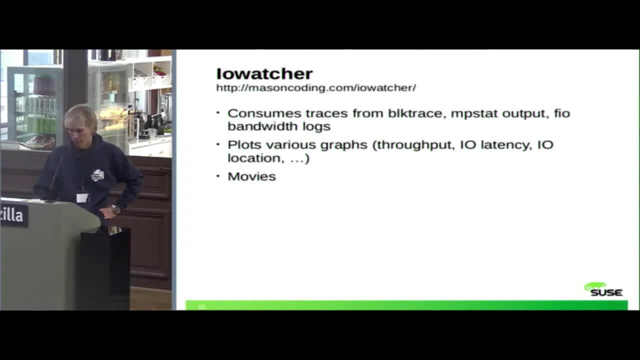 in the block layer. it can also consume mpstat output, which is showing some CPU utilization and so on. it can consume also output from FIO, which is a benchmarking tool, and it will. it can plot night graphs from that so it can show throughput latency and so on. I will show. 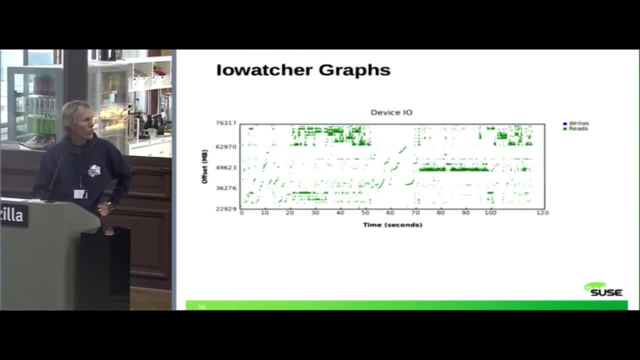 it in a moment. So this is the first type of the graph. on the x-axis you have time. on the y-axis, you have offset on the disk, so you can. this is actually the graph through the kernel tree. I've already captured and I was preparing the presentation. you can see we are seeking. 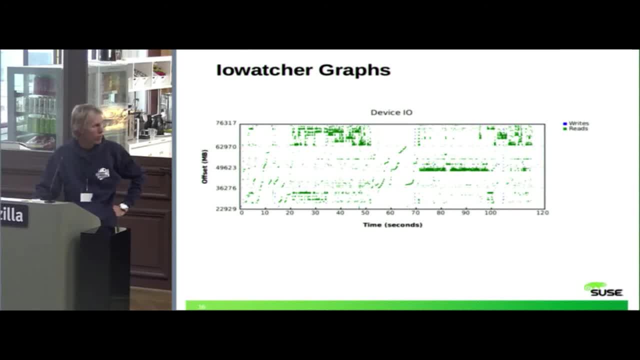 quite a bit over the all over the disk. it's mostly lead workload, naturally, as it is scrap. occasionally there are some bribes, but you cannot probably recognize it. You would have to take a magnifier glass to find them. they are a bright back of the updated. 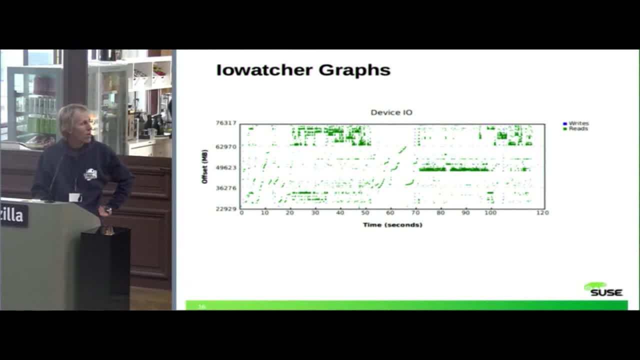 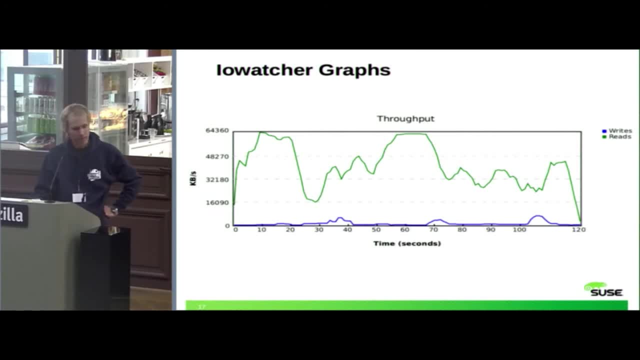 access time timestamps in the inodes. So that's first type of the graph. second type of the graph is a throughput graph, so you can see how the throughput goes when the test was running. and again for reads, for bribes: the blue line is bribes, green line is reads. 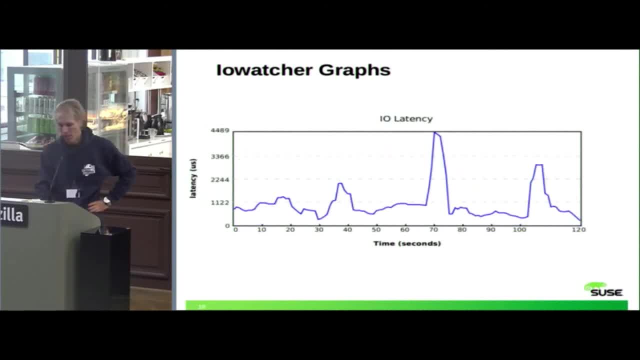 We have, Okay, Okay, So the IO latency, so its latency of average IO. this is again some rolling average. so we see the latency was mostly around one millisecond, with some peak up to four milliseconds, some, some around seventy seconds. 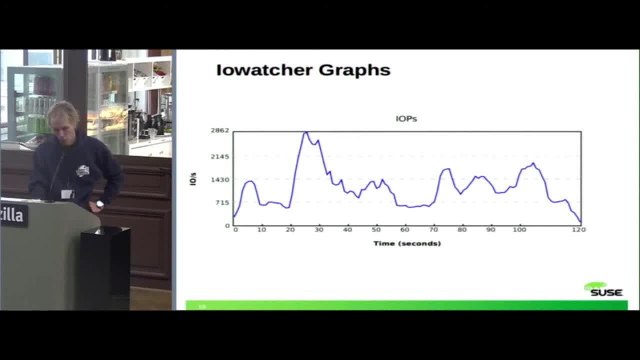 The number of operations per second. this is kind of similar to throughput, but sometimes it's better to look at throughput, sometimes that IO operations per second. it depends what you want to compute. Okay, And this is QDAP. Now you can, for example, notice that: so QDAP is the number of requests that are outstanding. 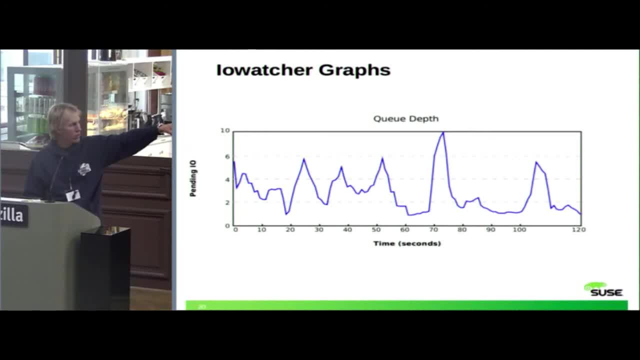 for the device and you can notice there is a peak around second seventy and then around second hundred, which kind of corresponds to the peaks in IO latency, so which is kind of what you would expect like when the requests are sitting in the queue. then obviously takes. 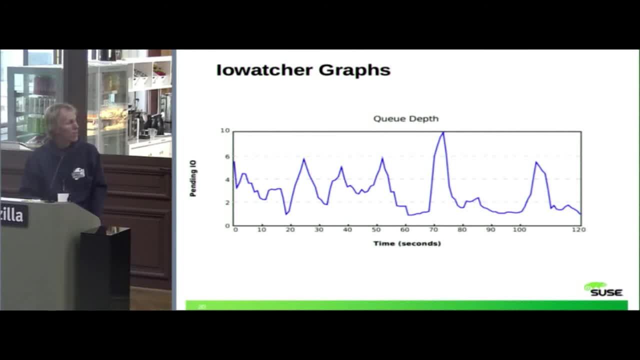 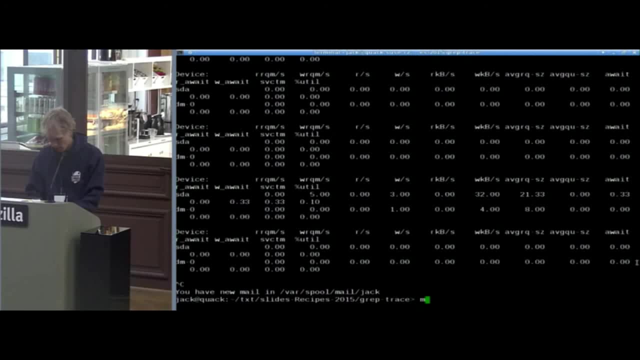 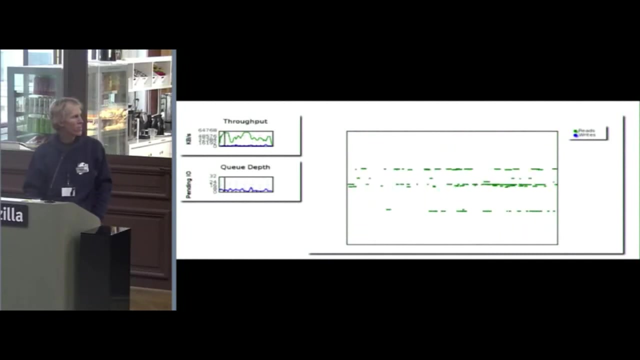 longer time, longer time to complete them. Okay, So the graphs aren't probably made up Now. movie time. So IO Watcher can also generate movies. So this one. So this is the movie IO Watcher can generate. 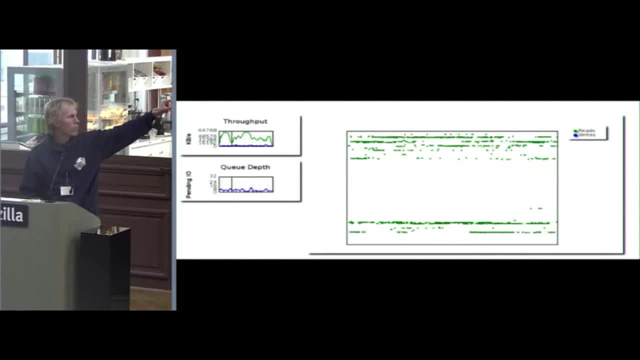 On the left you can see the throughput and the QDAP. I think we can choose different graphs there as well. Okay, So in the middle there are there are like sectors which are being accessed. Now the whole rectangle is actually a disk, so you have like more detailed mapping than 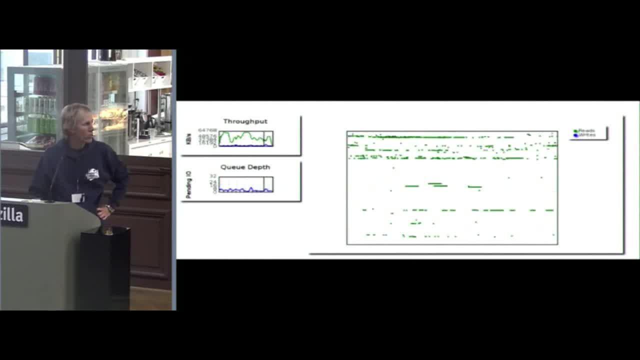 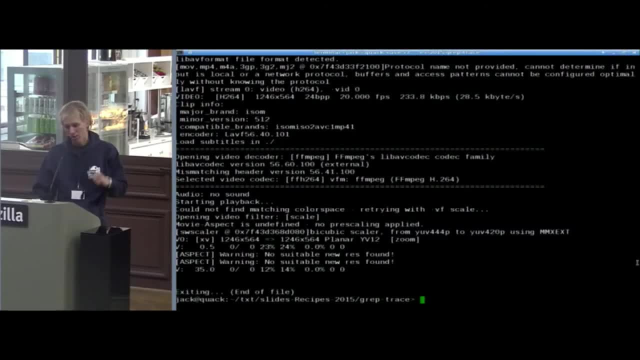 in the IO, in the static IO graph, because this is changing over time So you can see as we are going through this. occasionally you can see blue lines which are basically right back of the INode tables done in the background So it can generate movies. 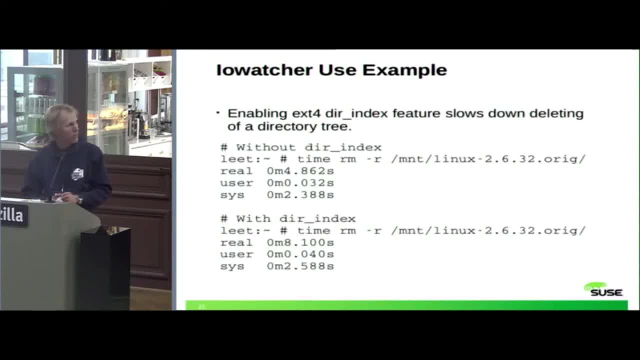 Like this And it can be useful for analysis, as we see in the next example. So I have observed some time ago that when you- and actually it's a known thing, though this is an example quite old- that when you enable their index featuring feature in EXT3. 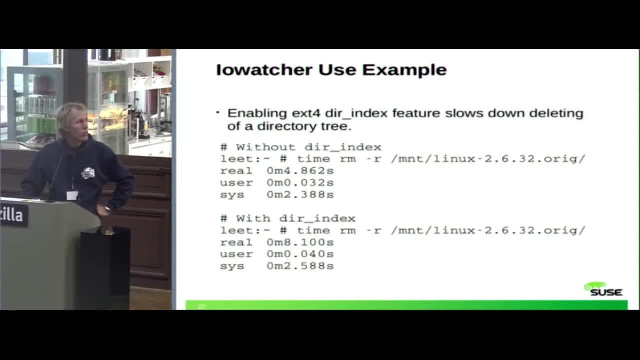 or EXT4, it slows down division of the directory tree. So the index feature is a feature which basically builds a bit And this is a B3 in each directory And this B3 uses some, So each name is actually hashed And then you have the B3 of these hashes. 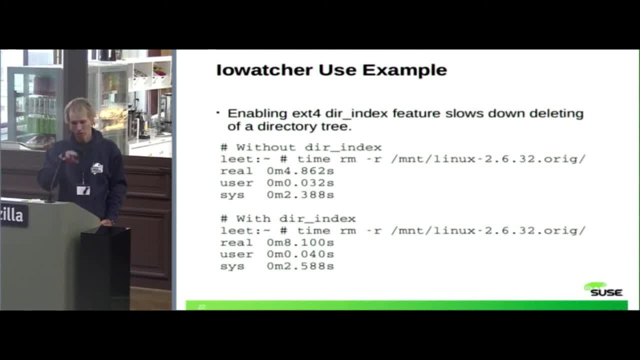 So the lookup can actually look up of the directory entry can work in logarithmic time. It just traverses the B3. And finds the entry quickly. So it's good for large directories And it can speed up lookup quite significantly. Okay. 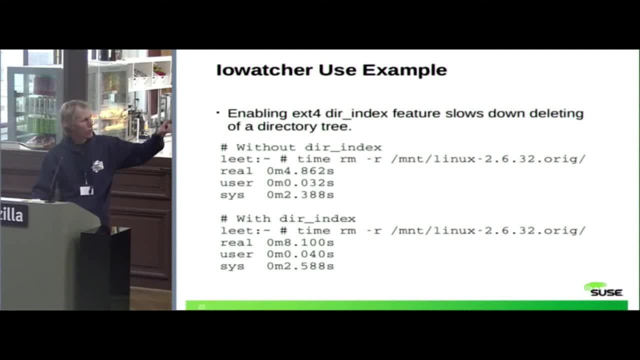 But when you are deleting the whole directory then you can see that without directory index you can delete kernel tree in bit under five seconds. But with directory index it takes over eight seconds. So it's noticeable slowdown. And now you may wonder why that is. 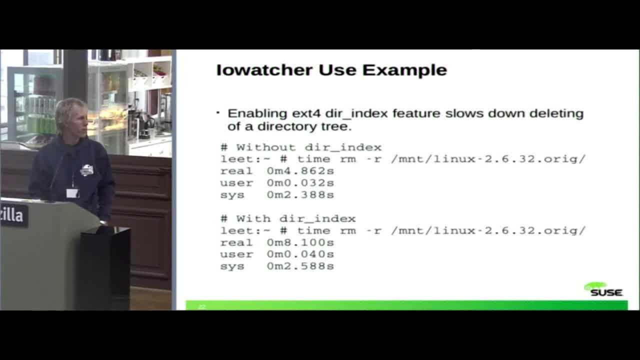 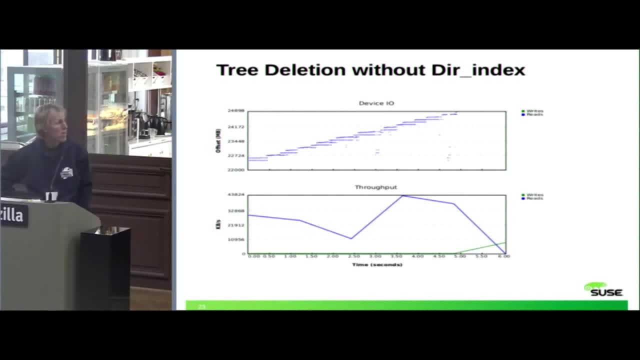 You know when this btree stuff should actually speed up things, not slow down. And so you capture block traces and then you plot them with IO watcher, And here you can see that actually the IO isn't really sequential, but we are seeking basically 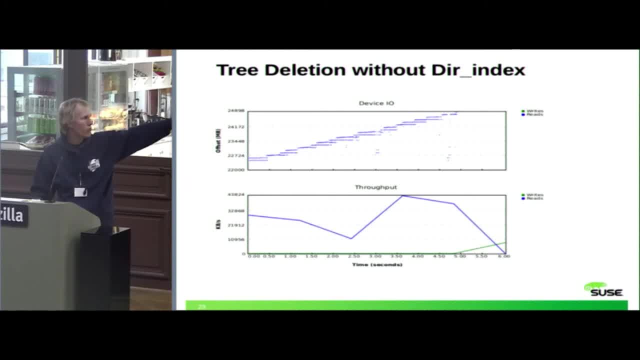 between two locations at each moment And the throughput is quite good, you know, 20 megabytes per second, which is for this workbook, like deleting lots of small files, a reasonable one. Now, if you look at the same trace, but without with the index feature, 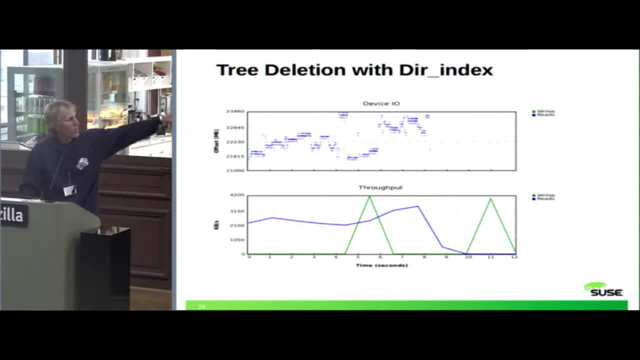 you can see we are seeking much more. We are seeking between more locations. you know the things are further apart. it's not really so nicely sequential So and throughput is much lower. So it's about order of magnitude lower, yeah. 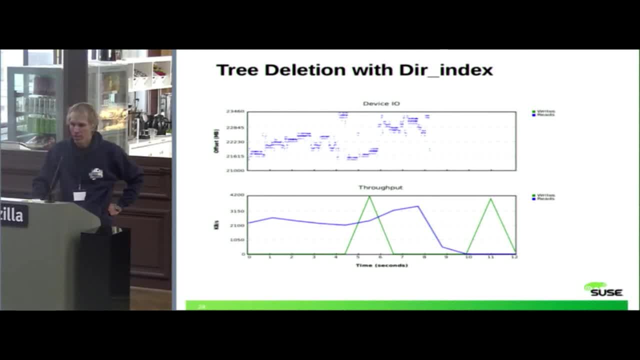 And the reason and when you look so you can see that really seeking is the reason why the removal is so slow. It's so slower And when you look into the what happens like in more detail, you will find out that the reason 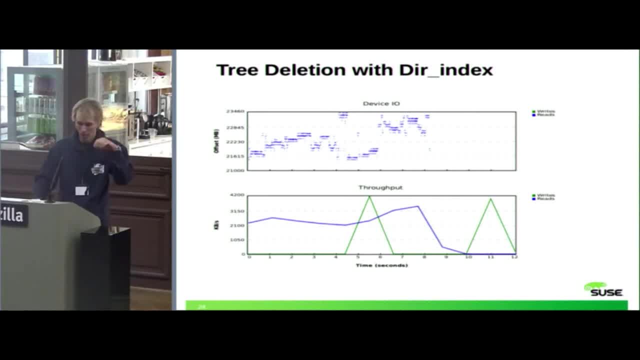 is that when you create directory, when you have the index feature disabled, then basically you delete the files in the same order and in which they were created And because when you are creating files you will place them one after another, then delete, and when you delete them. 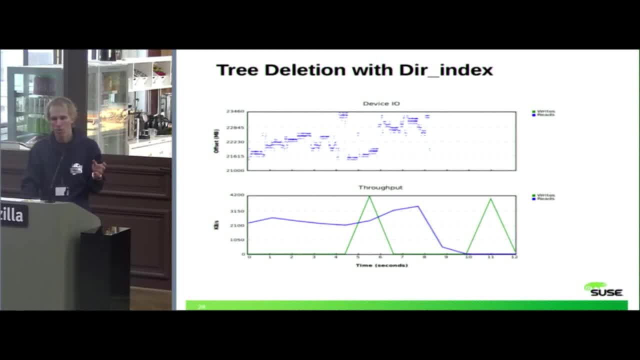 you will again delete them one after another. So you get mostly sequential IO, But with the index feature you will delete the directories in the hash order. So basically you can imagine like you would first sort the files by name and then start deleting them in this order. 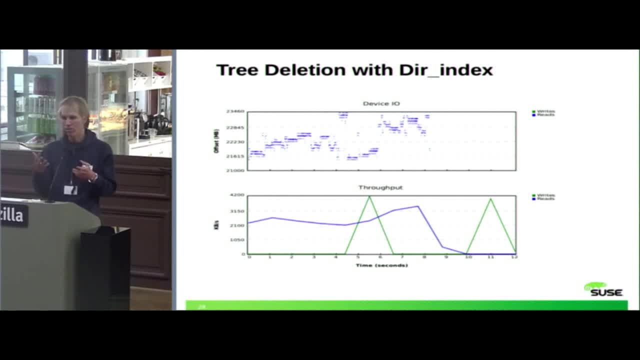 But this is basically random order with respect to the order in which the files were created. So, basically, you will delete file here, here, here, here here, and you are jumping between files, jumping between files in the directory, So the deletion isn't really sequential. 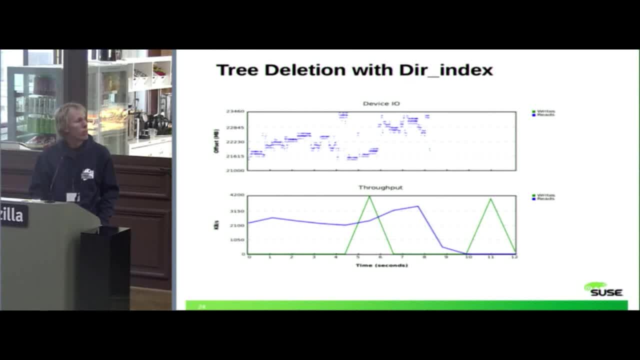 or is much, much more random than if you are doing it without this dir index feature. And the reason why it happens in the hash order is because, basically, rm first does read dir, which returns the entries in the hash order, and then it goes one entry after another and deletes them. 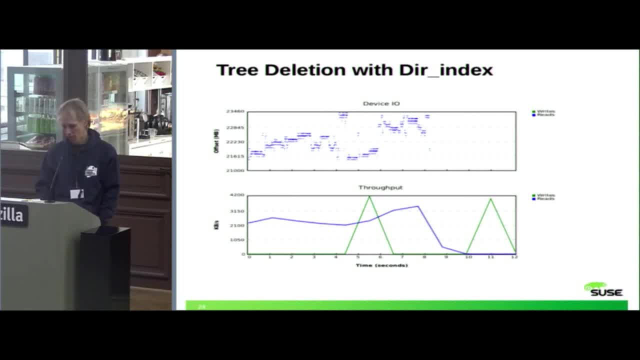 So it ends up deleting the inodes in the hash order of their names. So yeah, Yeah, Well, but you will also put the. so you know it depends. So with dir index, when it is mostly random, then maybe. 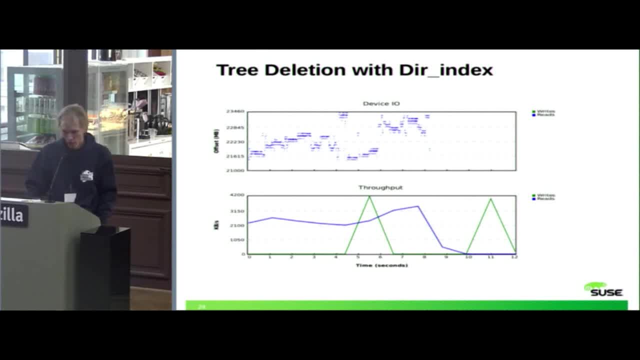 Yeah, but I guess in practice we you want anyway random right? Yeah, Yeah, Yeah, Yeah, Yeah, Yeah Yeah. So you have one that many processes in parallel, And so in the end I guess you won't gain performance from that. 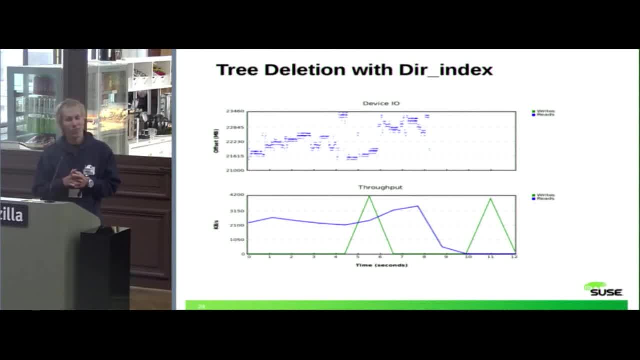 And you could possibly destroy the sequentiality that was previously in the workload. So if you would do this without the dir index feature, you would destroy the sequentiality of the removal. yeah, Because you will then delete like files from this directory.